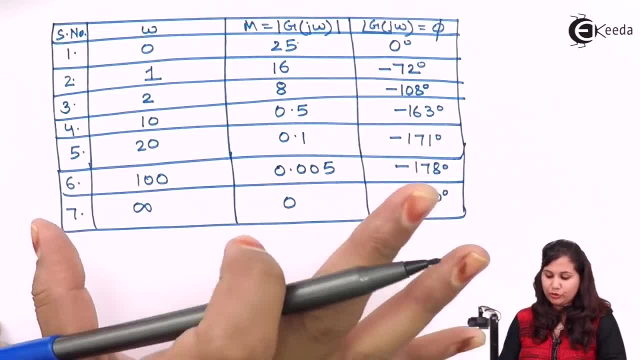 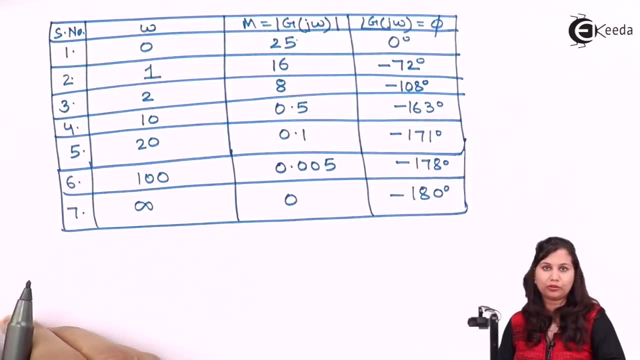 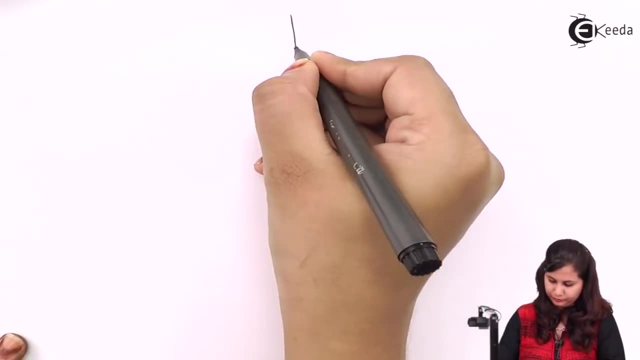 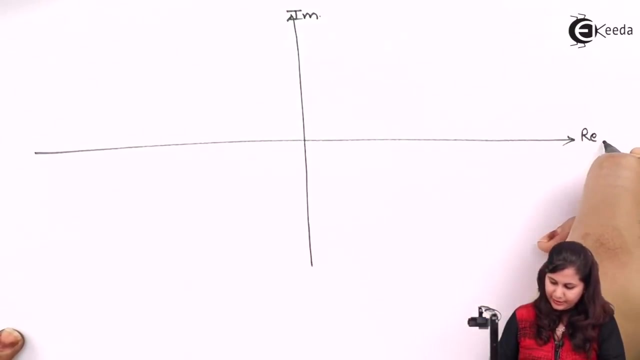 magnitude and the phase angle. now we are going to plot this magnitude and the phase angle on the polar coordinates, okay, so that we will be able to find out the polar plot of the system. this is our imaginary axis and this is the real axis. magnitude is plotted on this real axis. 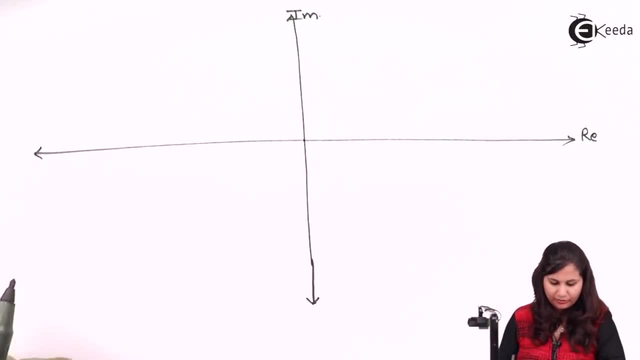 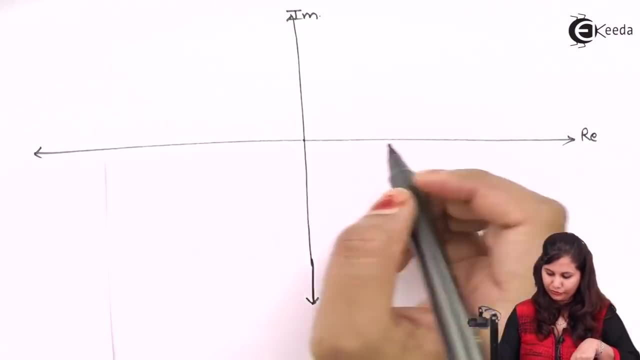 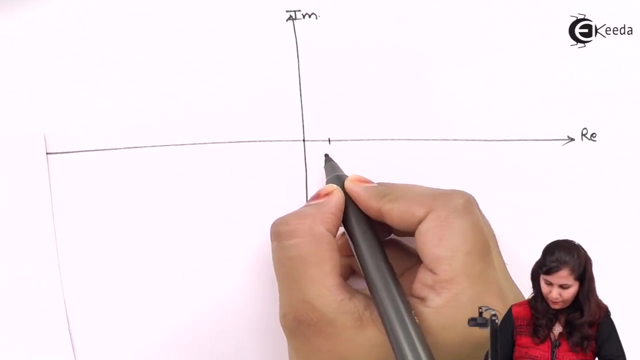 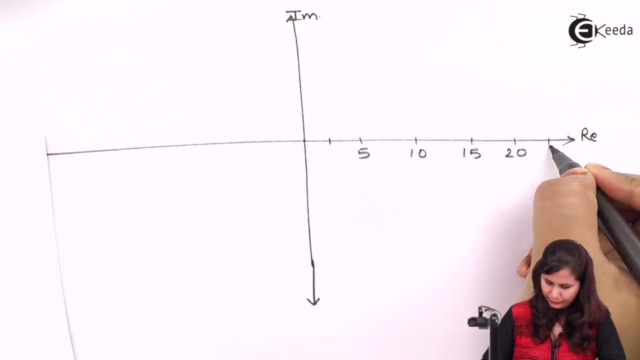 okay, so first we will draw. we have the magnitude as 25, 16, then 8, 0.5, 0.1. so we will divide this on. we have 5, 10, 15, 20, 25 okay, and this will be 2.5. this is 0. 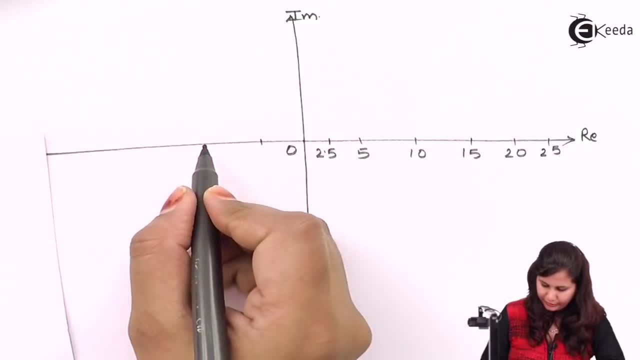 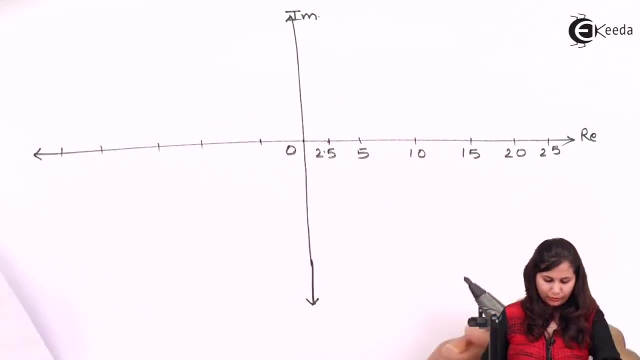 here also, you will divide 5, 10, 15, 20, 25. okay, now, when you can see that when omega equals to zero phase angle is zero degrees. so this is 0 degrees, this is plus 90 degree. this is minus 180 degrees, this is minus 90 degrees. okay, and whenever we plot the negative phase angle, 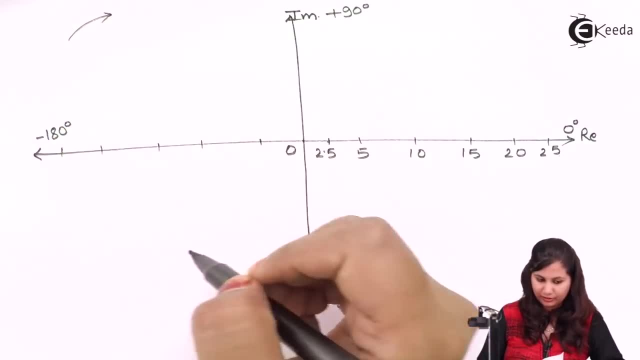 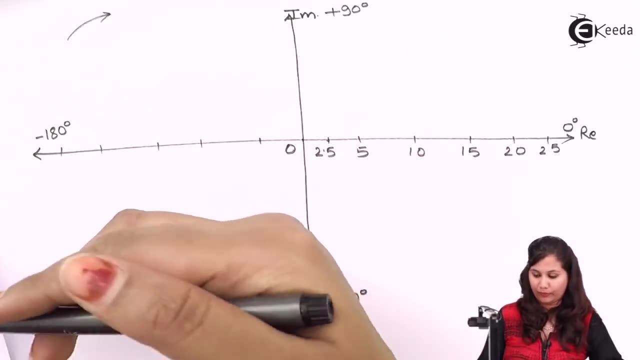 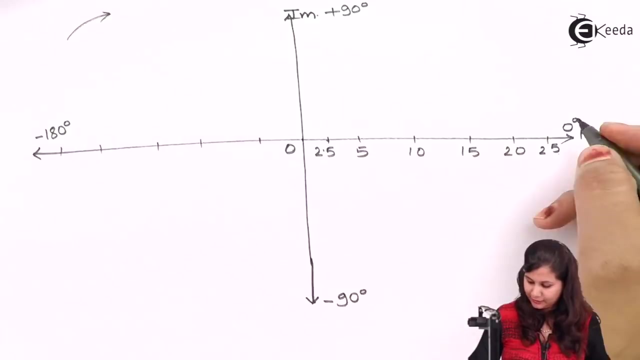 phase angle, it is measured in the clockwise direction in the polar plots. okay, and if the phase angle is positive, it will be measured in the anticlockwise direction. So for omega equals to 0, the magnitude is 25 and phase angle is 0 degree. so this is the point. okay, for omega equals. 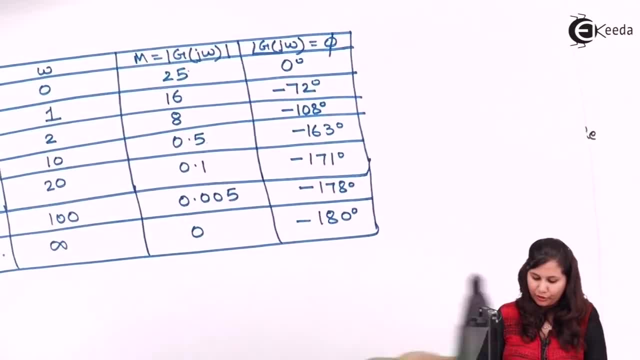 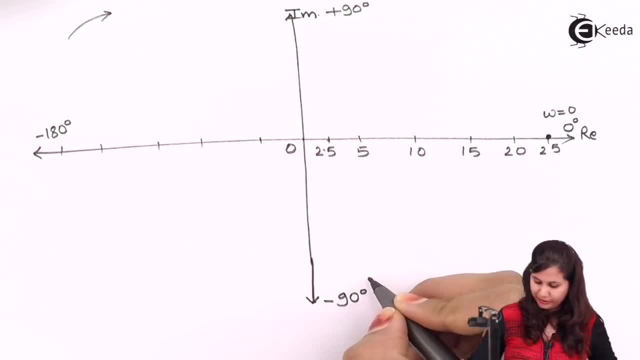 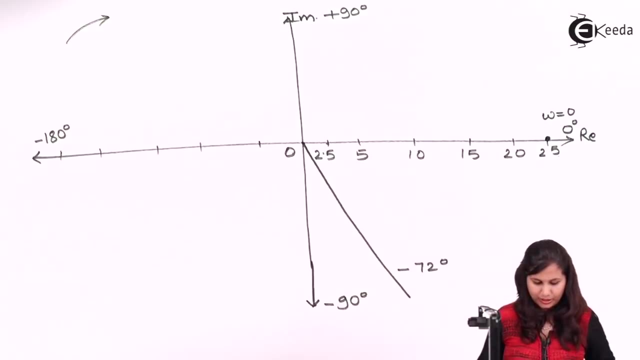 to 0.. Now, for omega equals to 1, the phase angle is minus 72 degrees. minus 72 degrees will be here. so minus 72 degrees, okay. and for omega equals to 2, the phase angle is minus 108 degrees. so it will be in this direction. 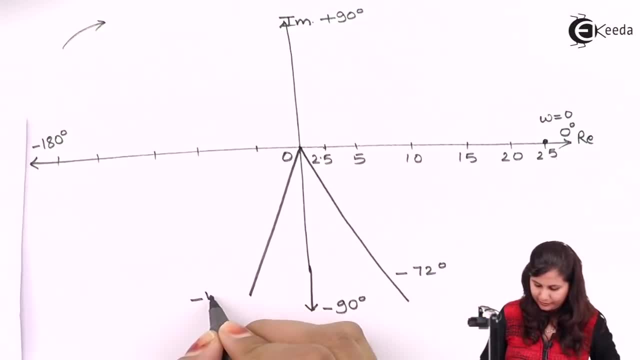 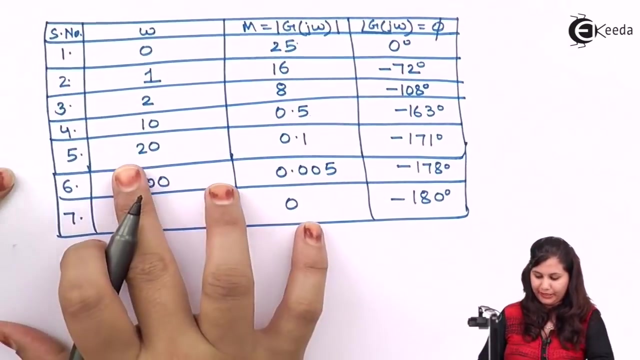 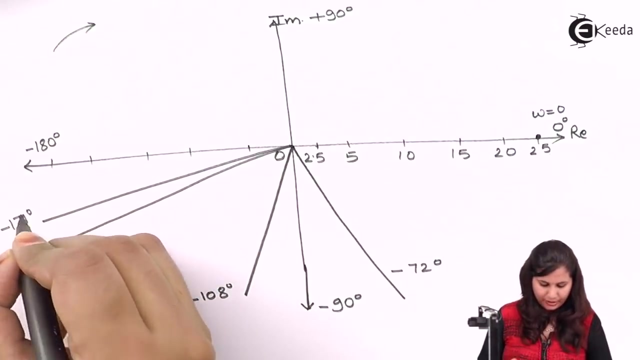 minus 108 degrees. for omega equals to 10. phase angle is minus 163 degrees, so it will be 163 degrees. then for omega equals to 20. phase angle is minus 171 degrees, so 171 degrees. then for 100 we have 178 and for omega equals to infinity. 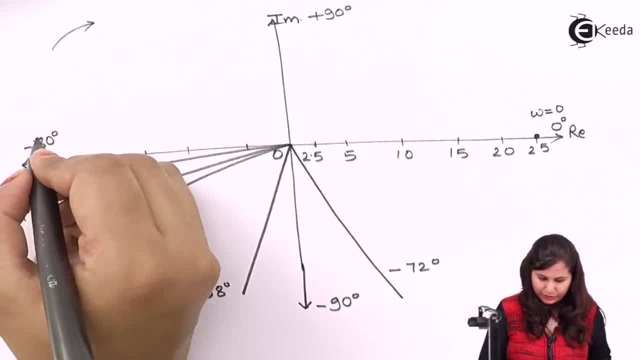 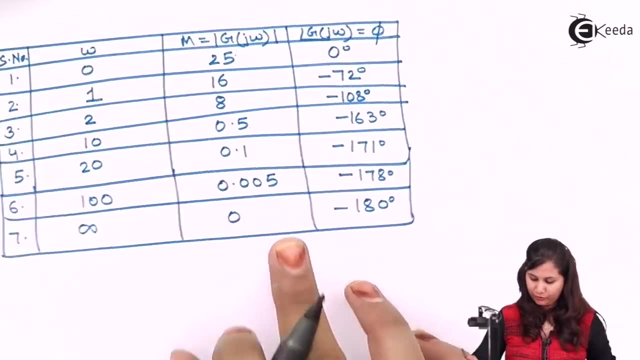 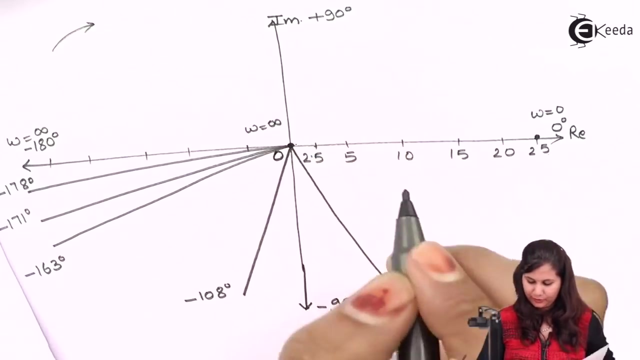 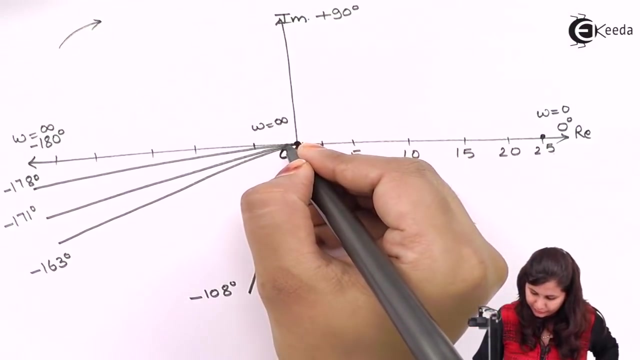 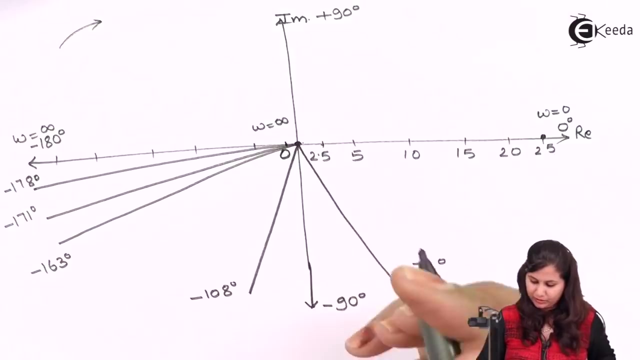 the phase angle is minus 180 degree, so it is for omega equals to infinity. now, at infinity, the magnitude is 0, so it is here omega equals to infinity and the value is 0. then for omega equals to 100 magnitude was 0, 0, 0.5, so it is somewhat here ok. for omega equals to 20, magnitude is 0.1. 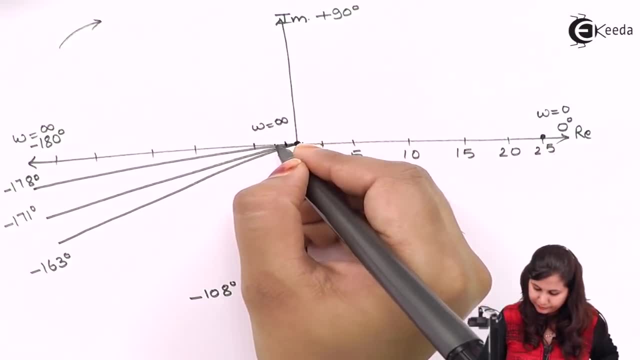 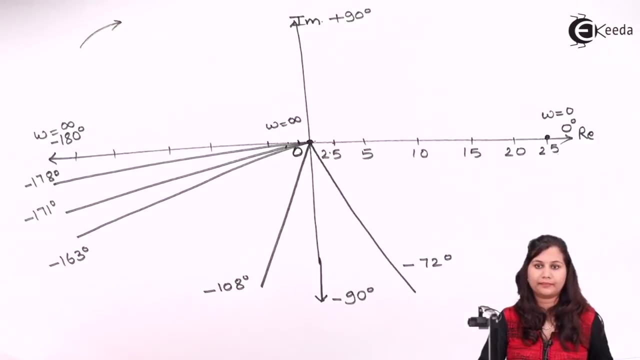 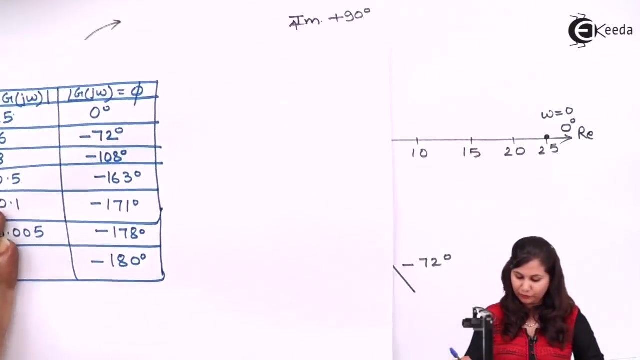 so 0.1 will be also somewhere here. so when we mark all these points, ok, and then. so for various values of the omega, we will mark the points. that is, for omega equals to 0,, 1,, 2,, 10.. For omega equals to 10, it is 0.5. 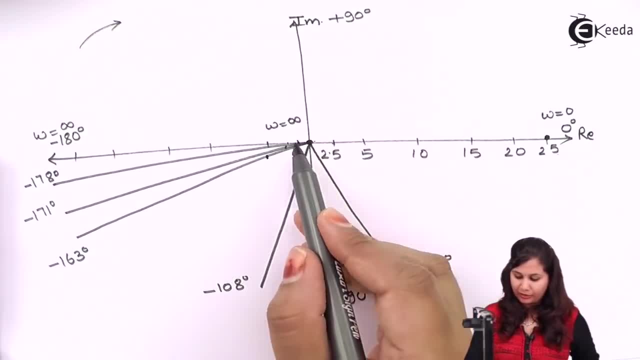 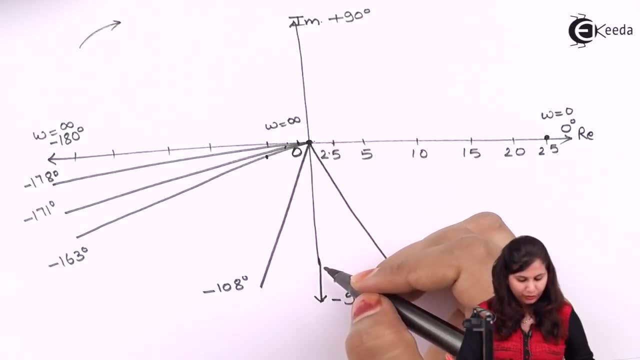 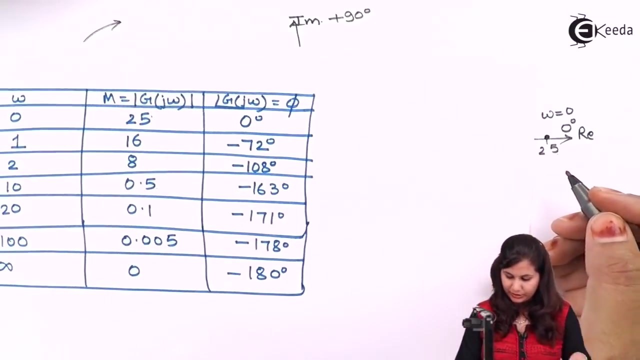 So it is here. Now we have marked all the points. Let us join these points so that we will obtain the Nyquist plot, For omega equals to 2, the magnitude is 8 and the phase angle is minus 108 degrees. So we will join these points. 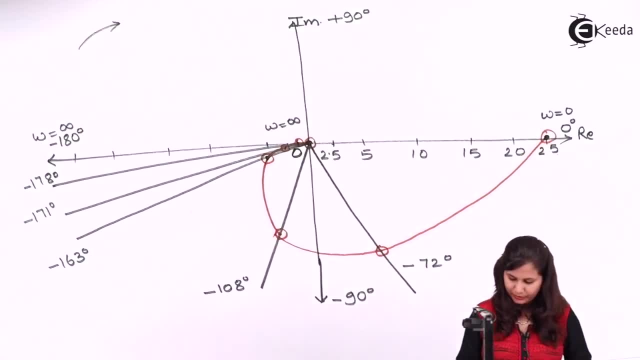 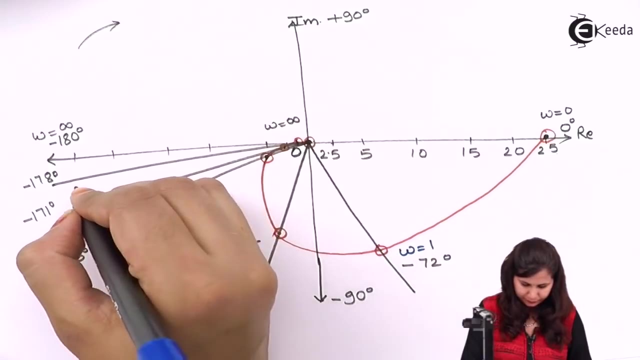 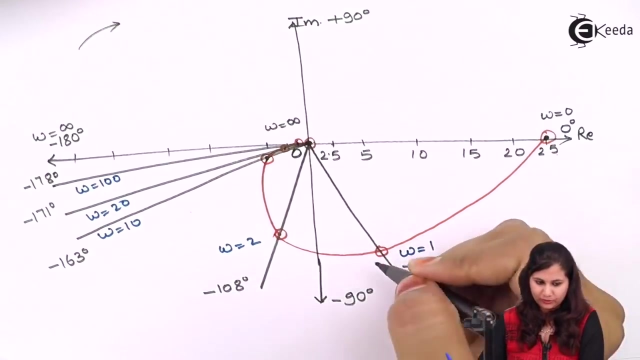 Okay, And write the frequencies over here. This is for omega equals to 0.. This is minus 72 degrees, is for omega equals to 1, omega equals to 2, omega equals to 10.. Okay, Write the frequencies over here and we have joined the points. Okay, And it is the. 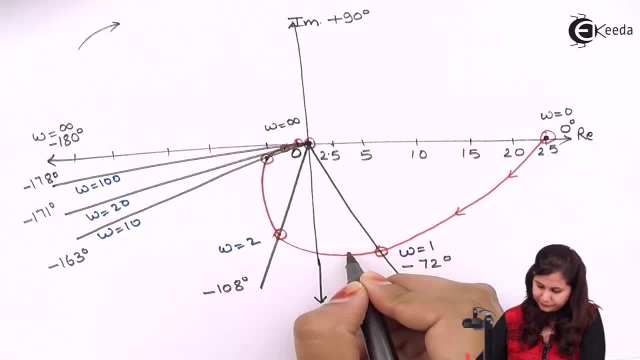 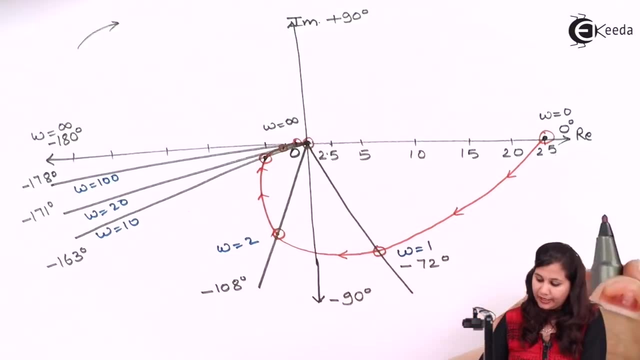 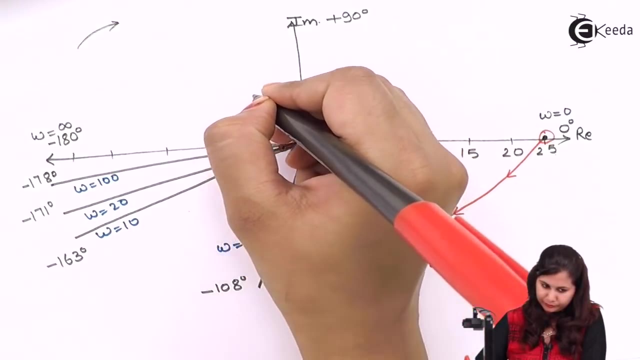 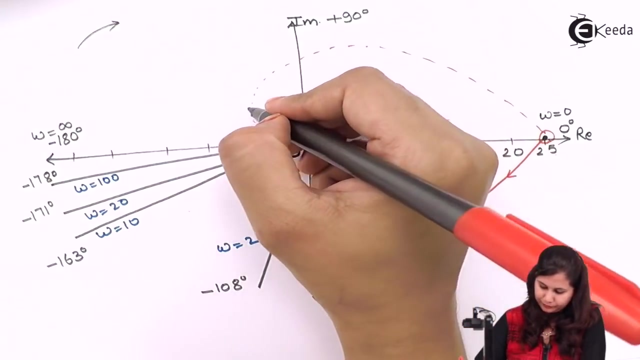 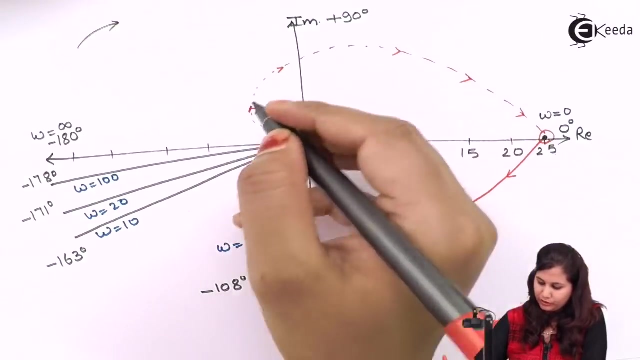 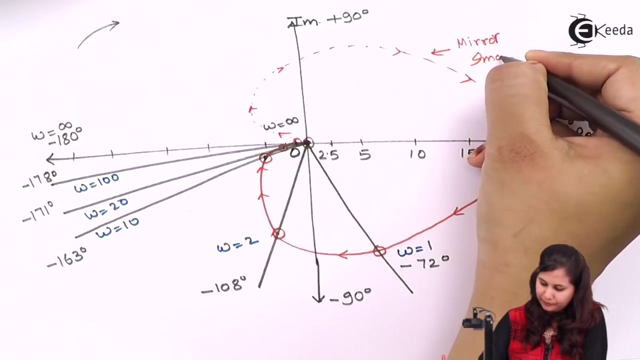 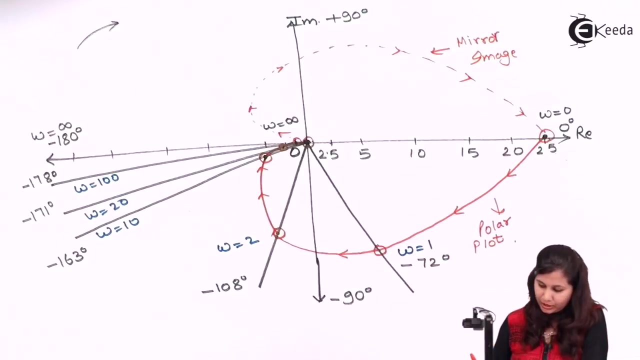 direction of the polar plot, starting from omega equals to 0 and terminating at omega equals to infinity. Now draw the mirror image of this plot. Okay, We have drawn. This is the mirror image of the polar plot. It is the polar plot of the system. Okay, Now let us see that. whether this point has 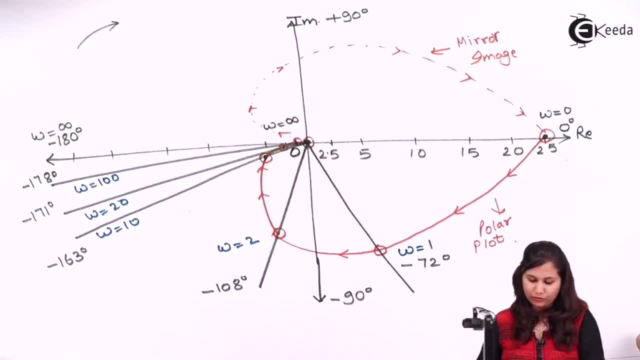 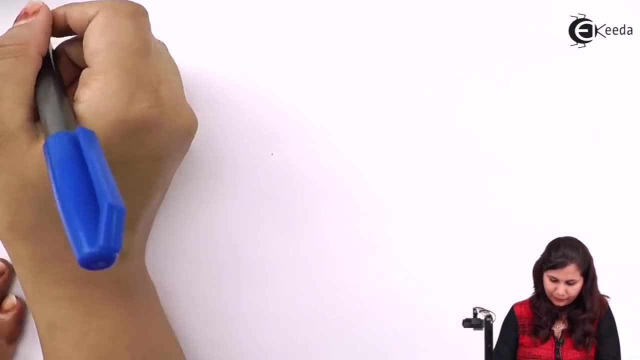 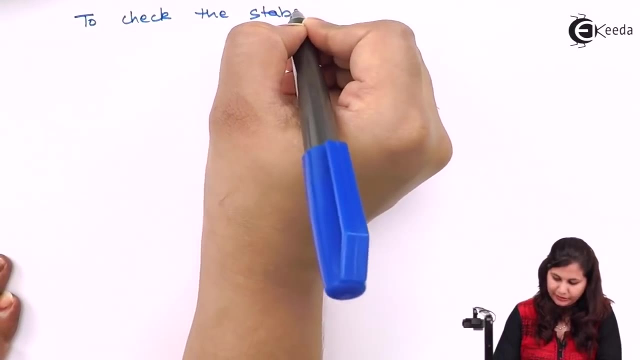 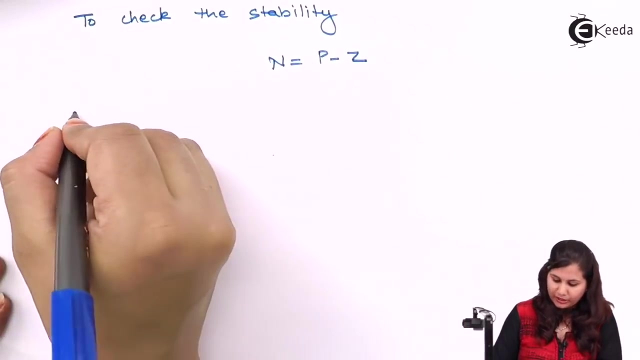 encircled the minus 1 plus j, 0 point, We have drawn the polar plot. Okay, Now our next step will be to check the stability. Now for stability check we will use the equation: n equals to p minus z. n is what. 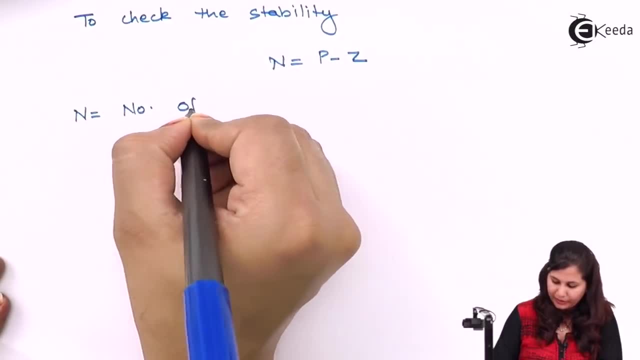 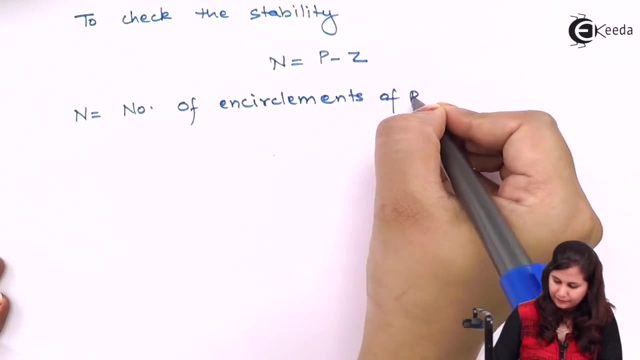 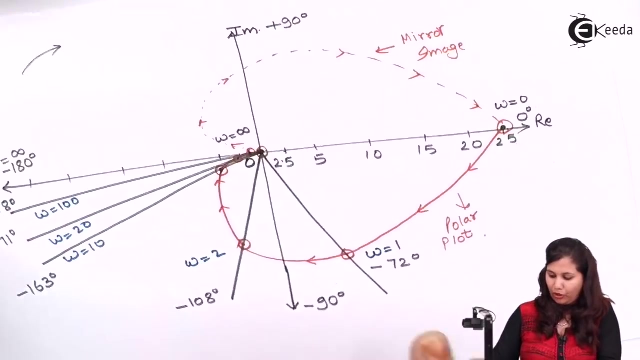 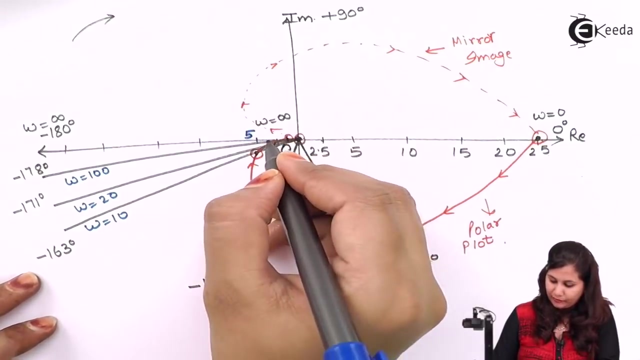 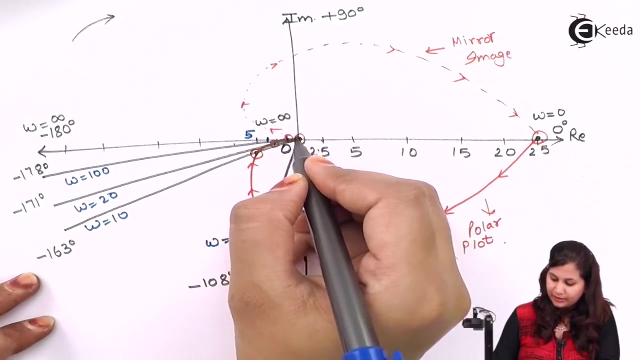 It is the number of encirclements of the point minus 1 plus j 0.. Now here this plot. it is not encircling the point minus 1 plus j 0. This is 5.. Okay, And 1 is here 0,, 1,, 2,, 3,, 4, 5, we will divide The point. it is the plot. 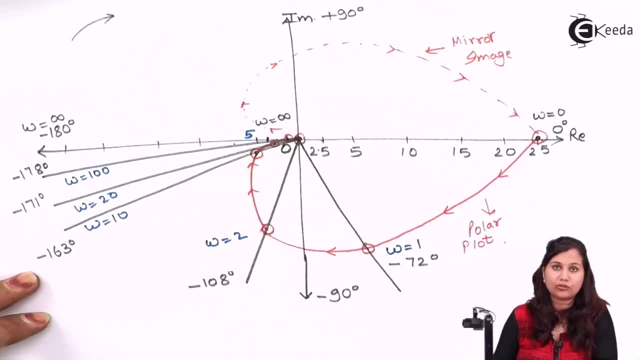 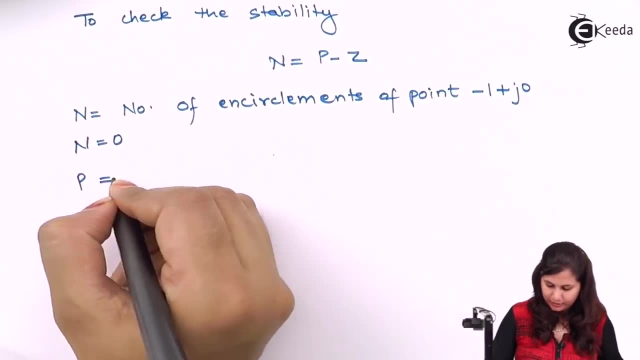 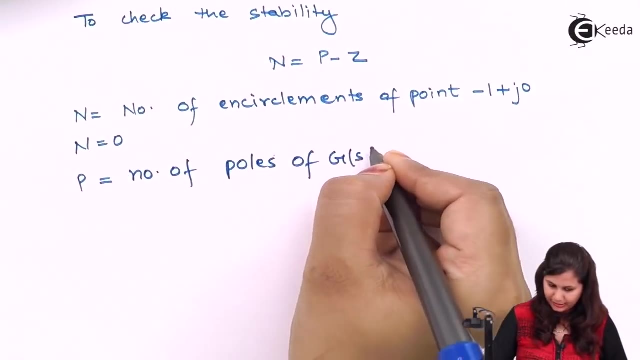 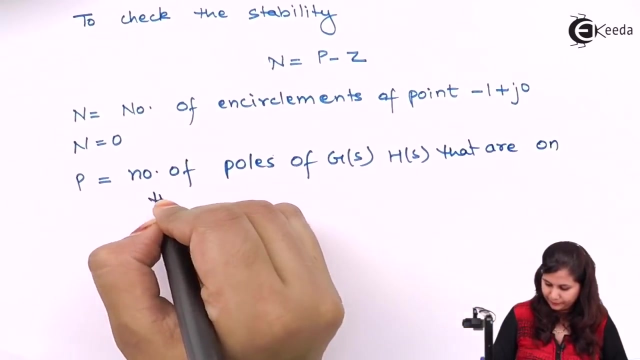 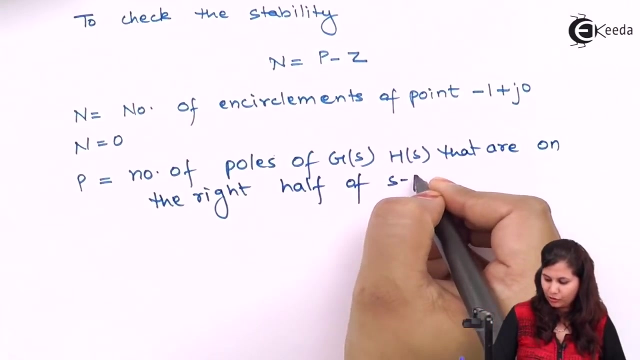 it is not encircling this. minus 1, plus j, 0 point. Okay. So n will be equals to 0.. Now p, it is the number of poles of gs, hs, Okay, That are on the right half of the s plane. So here, no pole is on the right half. 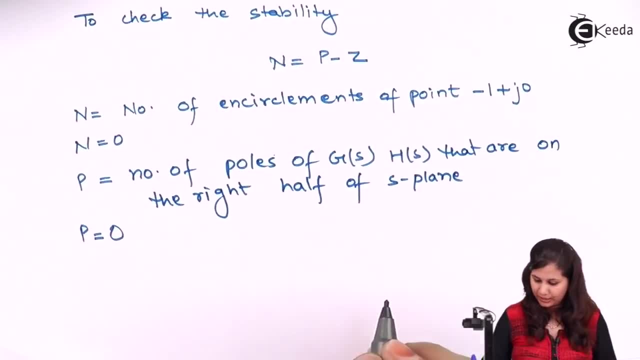 of the s plane. So p is equals to 0, because our transfer function was gs equals to 50 upon s plus 1, s plus 2.. So we have only two poles: s equals to minus 1, s equals to minus 2, and both these poles they are lying on the left hand side, So no pole is on the right half of the s plane, so p will be equals to 0. 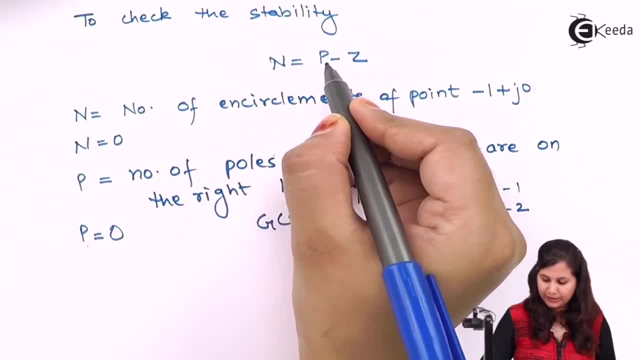 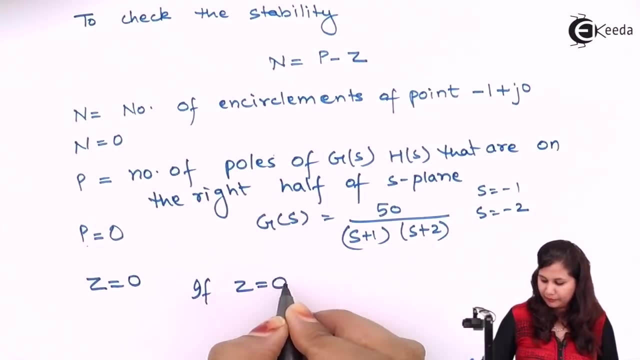 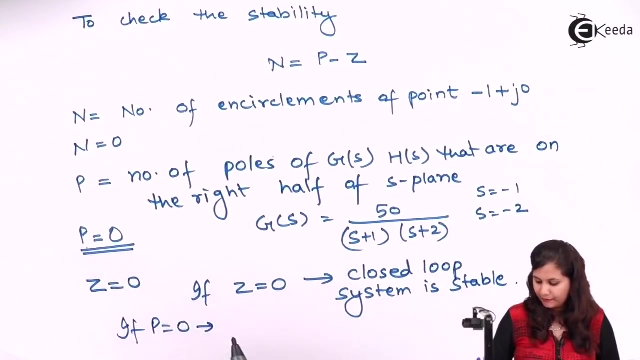 Now from this equation: n is 0, p is 0, so z will be 0, and if z is equals to 0, it means that the system, closed loop system, is stable. Now here p is also coming out to be 0. So if p is equals to 0, then we can say that open loop system is stable. 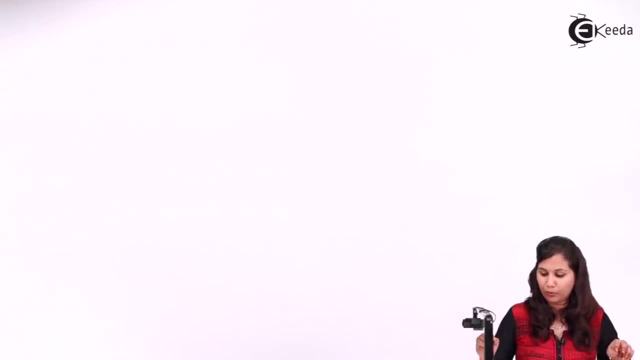 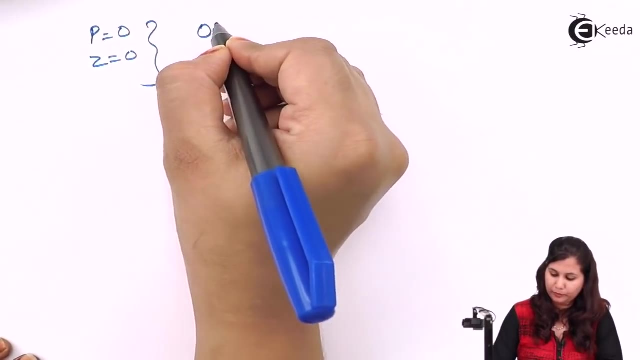 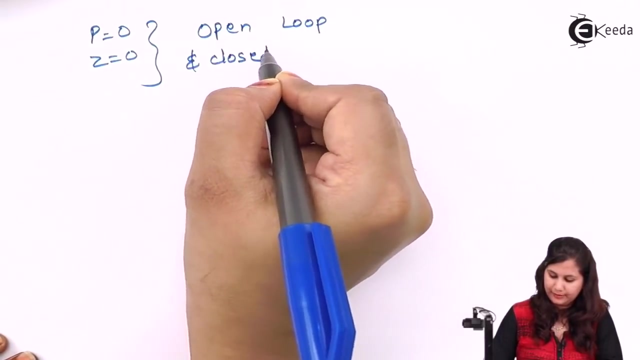 So for this transfer function we can say that both the p is equals to 0 and p is equal to 0.. So for this transfer function we can say that both the p is equals to 0 and p is equal to 0.. z equals to 0, so both open loop and closed loop system is stable. 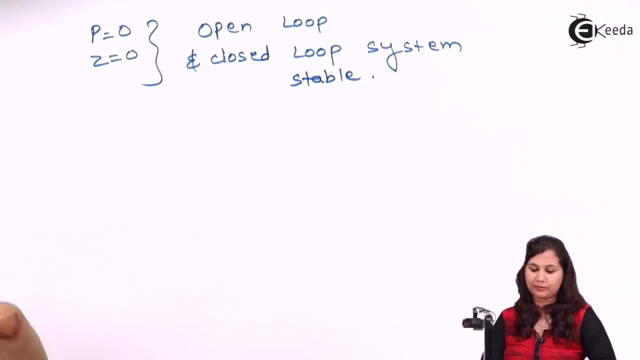 Okay, that is, both open loop stability and closed loop stability is present for this system. So whenever we want to have any question on the 9th Now we will check the Nyquist plot first we will put s equals to j, omega in that transfer function and then we will obtain the magnitude and the phase angle conditions. 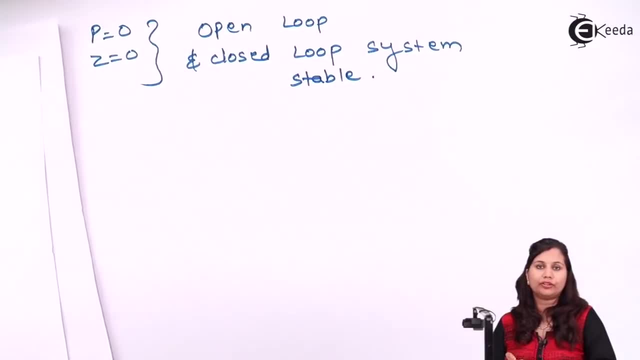 We will draw a table varying the value of the frequency from 0 to infinity. then we will draw the polar plot and from the polar plot we will draw the mirror image of that polar plot, so that we will be able to got the Nyquist plot of the system. 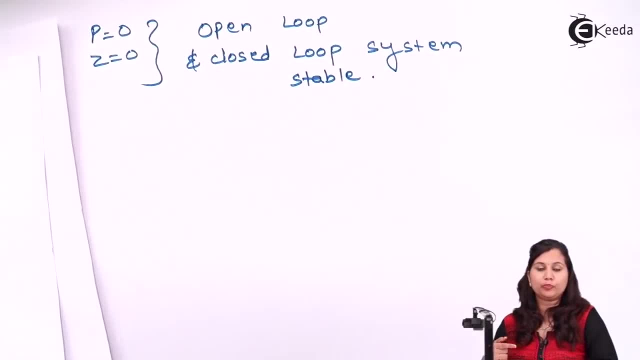 Now we will check that n equals to p minus z. we will use this equation to check the stability. we will observe the number of encirclements of the minus 1 plus j- 0 point and then we will comment on the stability of the system, whether the open loop system is stable or the closed loop system is stable or the system is overall stable. 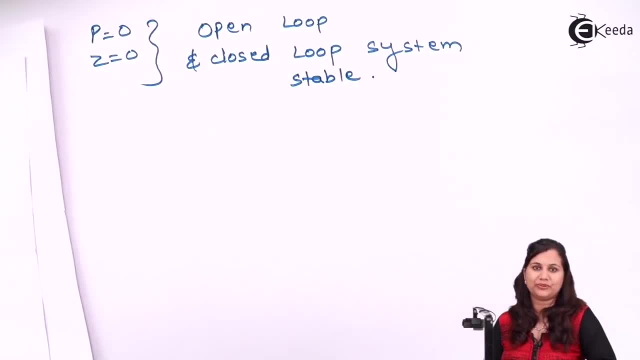 Okay, so I hope this problem is clear to you. Thank you. 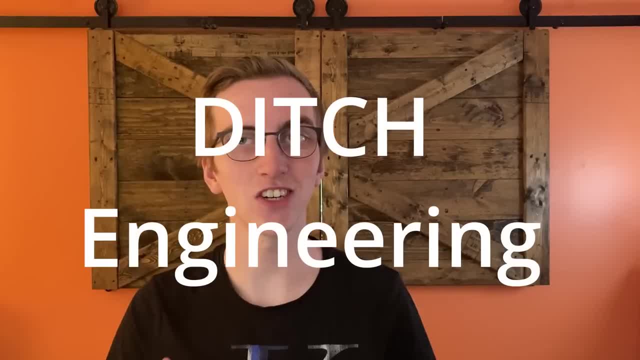 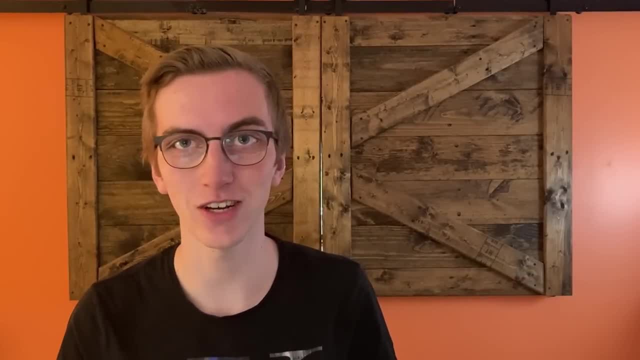 75% of engineering graduates end up ditching engineering right after graduation. What's up everyone? it's Oliver. Today I'm going to be talking about why so many engineering graduates don't end up working in engineering. If you've ever been on the dark, 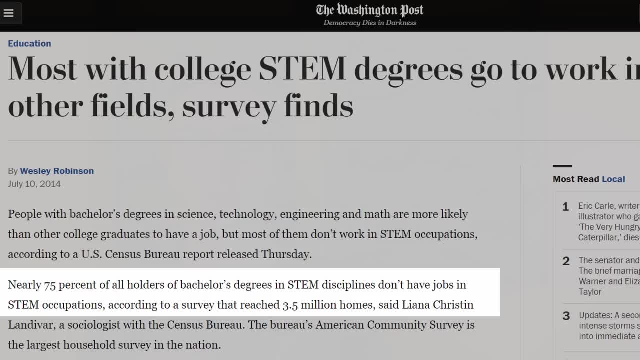 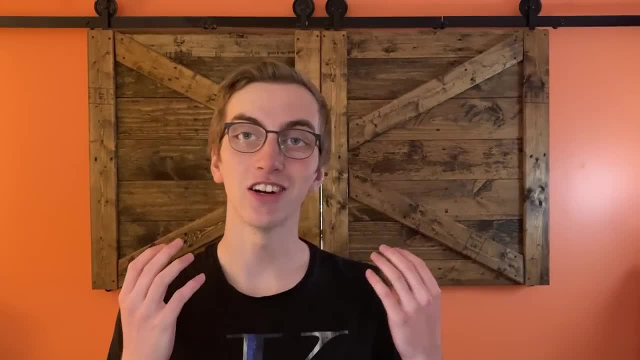 web of engineering. you've probably seen a statistic just like this one many times before. But why is it that so many engineers don't end up working in their field of study? Well, there are a few common explanations for this. One of the common ones you might hear from students: 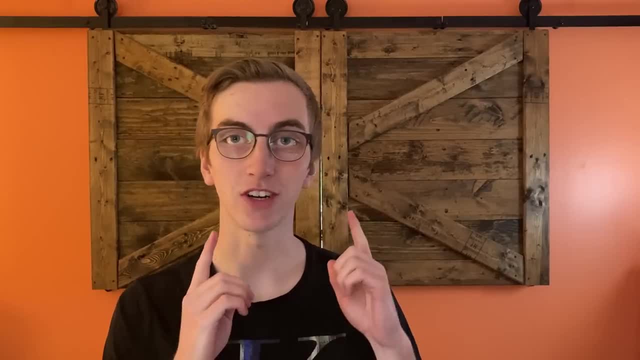 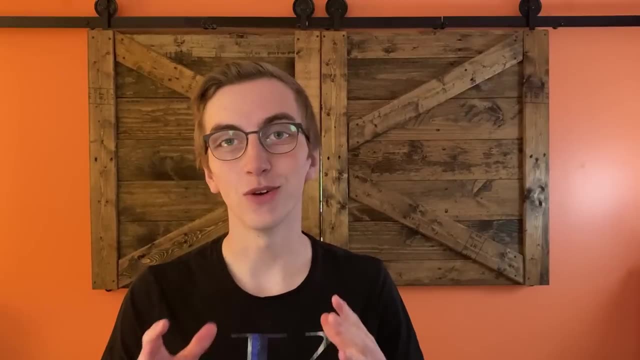 is that they can't find a job in their field. But if you were to go to the employers and ask them if they have job openings, they would often say that they have a hard time filling these spaces. So there is clearly a disconnect between the way that engineers are looking for jobs and 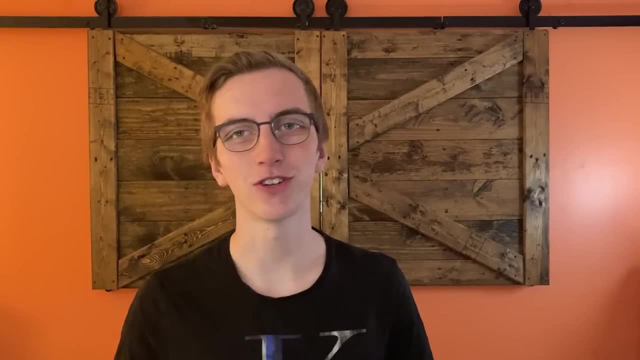 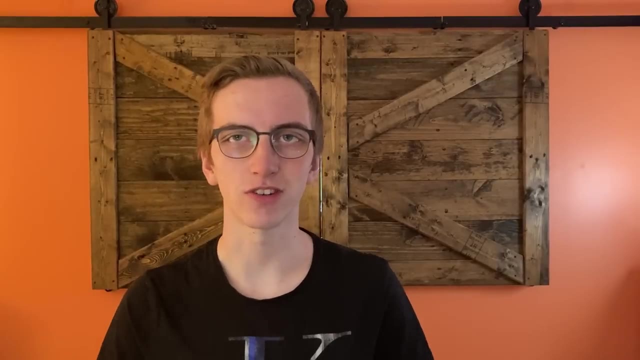 the way that employers are hiring for jobs. However, I'm sure you can figure out that this tiny discrepancy isn't enough to cover a gap of 75%. So the next logical step would be to say: are we graduating too many engineers? And the quick answer: